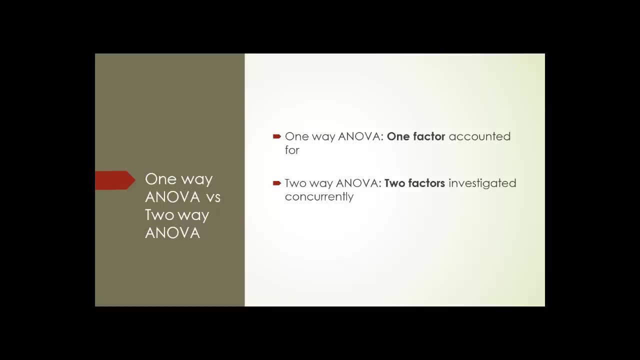 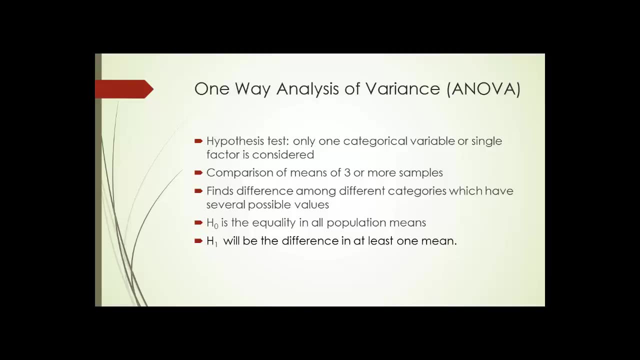 The experiment involves multiple variables. A one-way ANOVA involves a hypothesis test where only one categorical variable or single factor is considered. It's a comparison of means of three or more samples. If it were simply two samples, you would use a t-test. 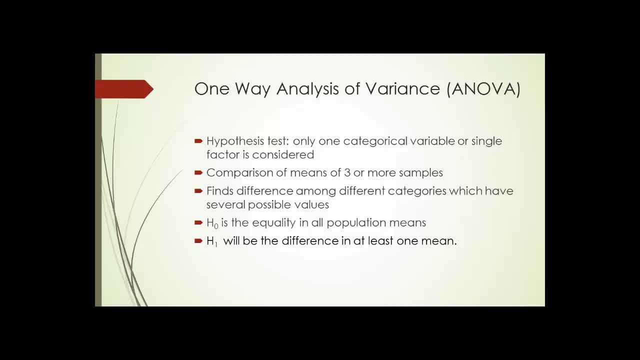 It finds the difference among different categories which have several possible values. values and a null hypothesis is that the equality in all the population means, and a directional hypothesis is that there will be a difference in at least one mean. This is commonly used by educational researchers, as well as in 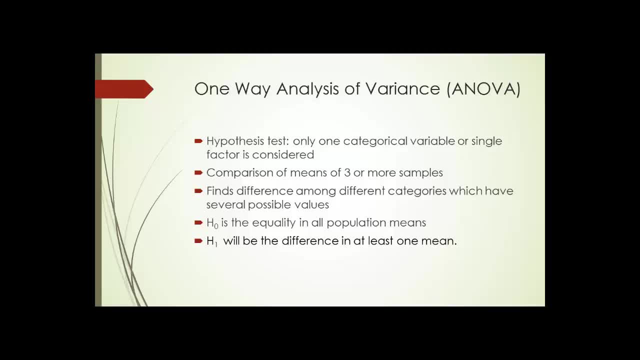 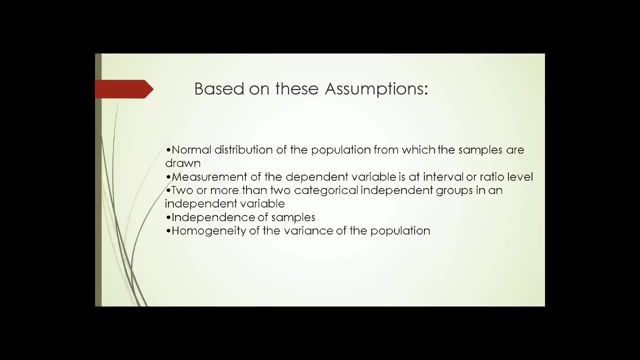 other fields, as we've already mentioned, in business, psychology, etc. There are several assumptions inherent to ANOVAs. First, normal distribution of the population from which the samples are drawn. Second, measurement of the dependent variable is at an interval or ratio level. Third, 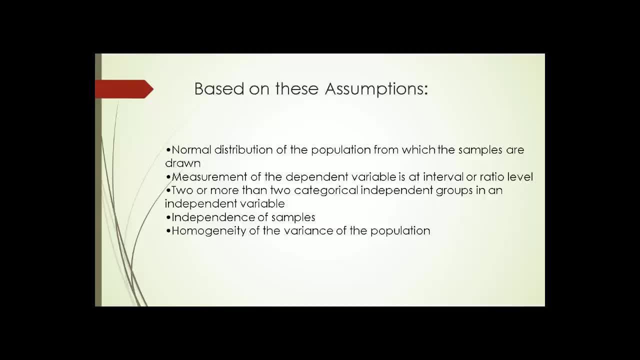 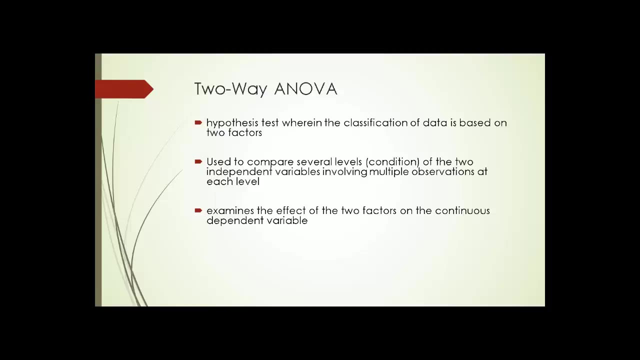 two or more than 2 gated coracle independent groups in an independent variable. Fourth, independence of samples. and fifth, homogeneity of the variants of the population In a two-way ANOVA, as its name signifies, a hypothesis tests wherein the classification of data is based on two factors. 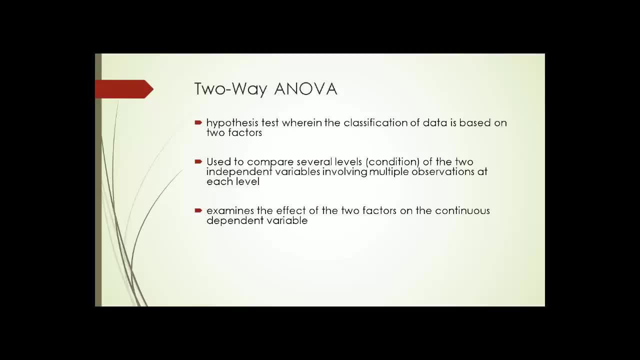 For instance, the two bases of classification for the sales made by the firm on: the first on the basis of sales by the different salesman and second by sales in various regions. It is a statistical technique used by the researcher to compare several levels of the two independent variables, involving multiple observations at each level. 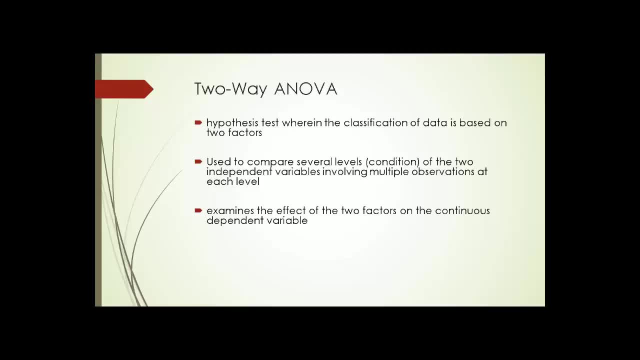 Two-way ANOVA examines the effect of the two factors on the continuous dependent variable. It also studies the interrelationship between independent variables influencing the values of the dependent variable, if any, And it involves two factors. It involves a hypothesis test wherein the classification of data is based on two factors.